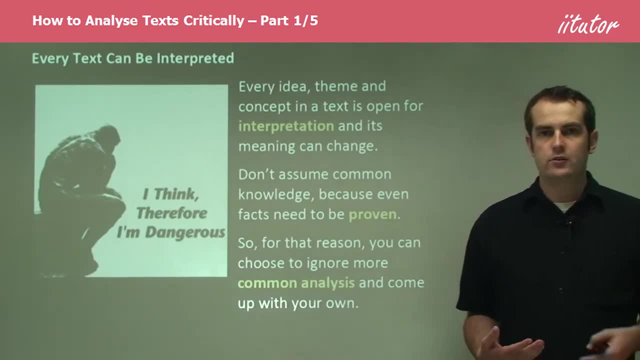 and really come up with your own. So you don't necessarily have to stick to the tried and true methods of analyzing a particular text. So if you're looking at a romance story, you don't have to necessarily say it's a romance story, so I have to talk about. being about love You can talk about. 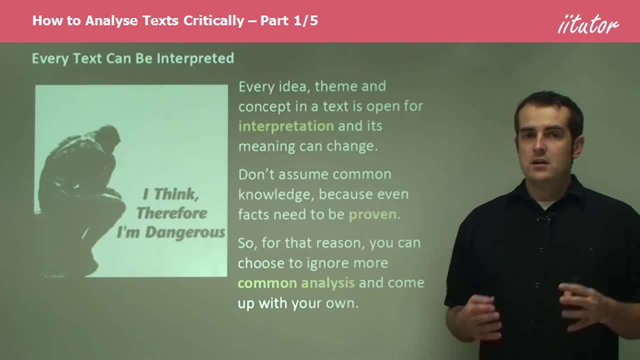 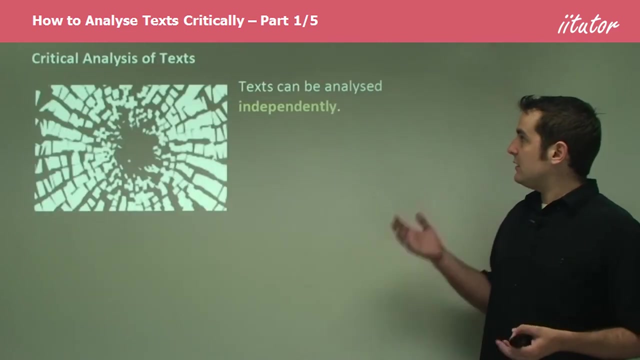 a lot of other things which may be important to the text and may contribute just as much to its meaning as love does. So there's not necessarily a common ground on how you need to analyze a text. It isn't purely up to you. Now, as I said, texts can be analyzed independently, which means they can. 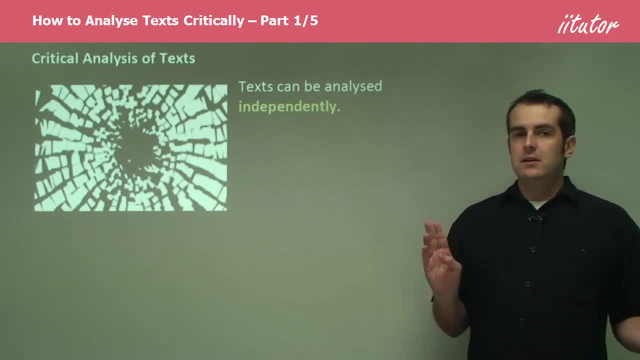 be analyzed independently, not just by you, but they can be analyzed independently of their context and by of their offer as well, which basically means that you are analyzing it, not off what someone else wants or by the opinions of a lot of different people. You can analyze it. 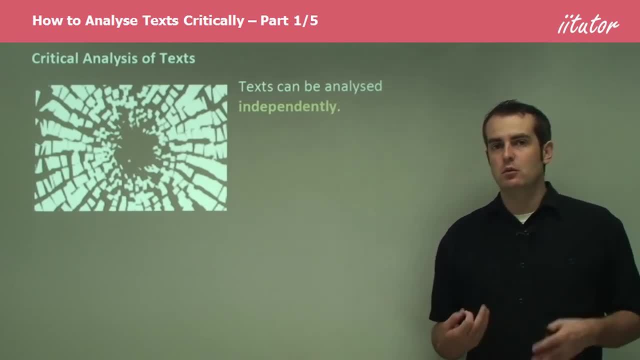 purely on what you think And really in English. that's what we're trying to get you to do is to analyze it in your own words, in your own voice and using your own arguments. I mean, if we wanted you to use someone else's argument, we'd get them to write it, but that's not what we want you to do. 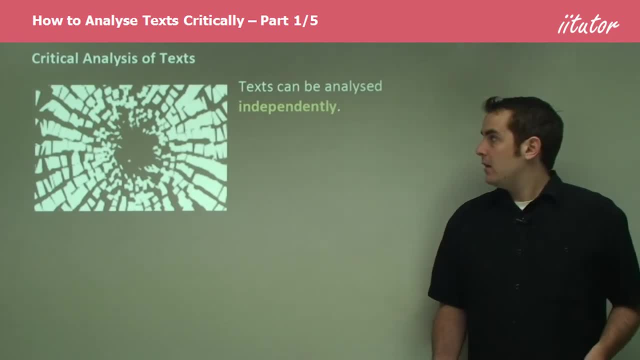 We want it to be about you, So what you can do Now. there is no set consensus on how you should analyze a text, only that you are able to justify the how and why in your argument. So in other words, you must be able to prove it. Now you can use your opinion. 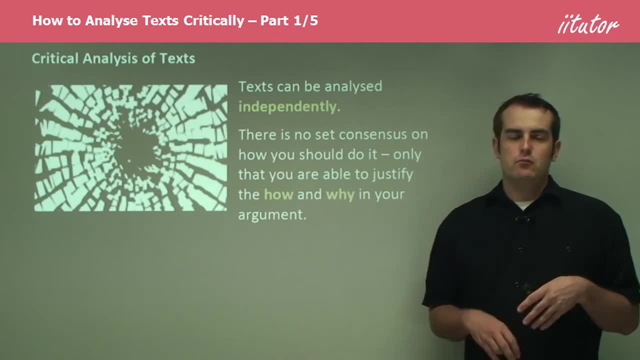 all you want, but you need to be able to prove it and you need to write it in such a way where you're using objective reasoning, In other words, that you are writing about in an objective kind of way, you're not putting your own personal opinion in there or, basically, you're not taking it personally. 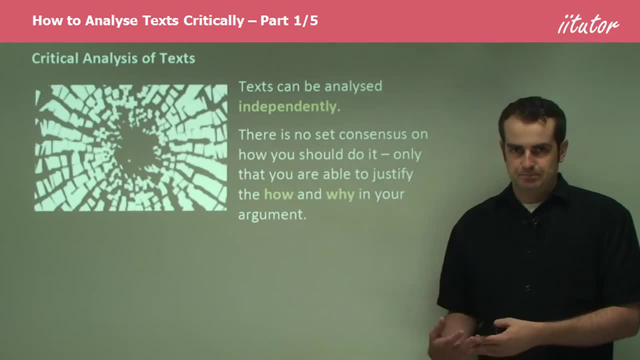 what it's trying to do, but you are including your opinion in such a way that you're talking about what facts are important to the overall meaning in the text. That's your opinion, but you're writing about in an objective way. I know it doesn't really make sense. 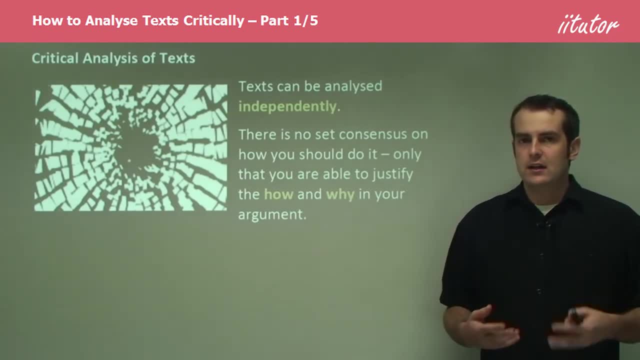 but when you're basically writing an essay or writing any sort of response requiring critical thinking, you need to just do more than provide your opinion. You need to be able to back it up. Now, being able to back up something with facts is more objective than it is subjective.